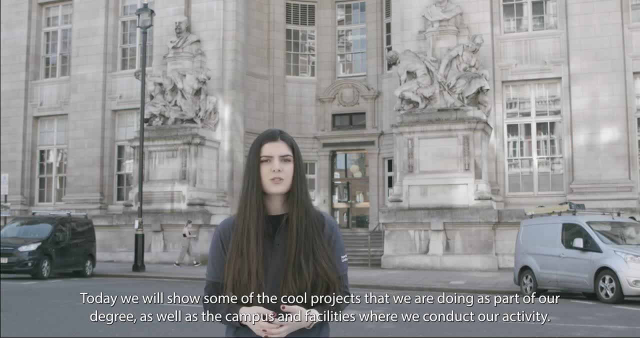 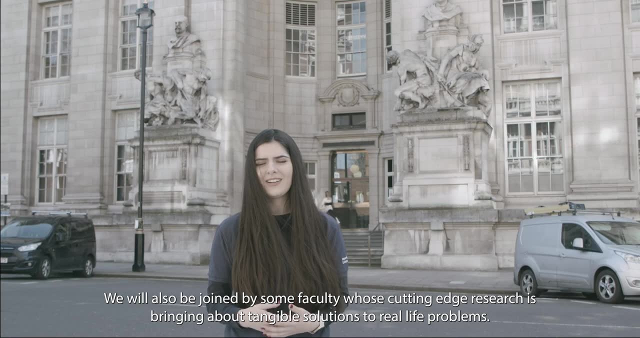 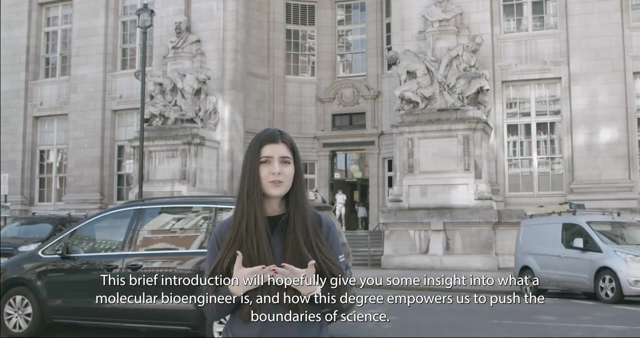 cool projects that we are doing as part of our degree, as well as the campus and facilities where we conduct our activity. We will also be joined by some faculty whose cutting-edge research is bringing about tangible solutions to real-life problems. This brief introduction will hopefully give you some insight into what a molecular bioengineer is and how this 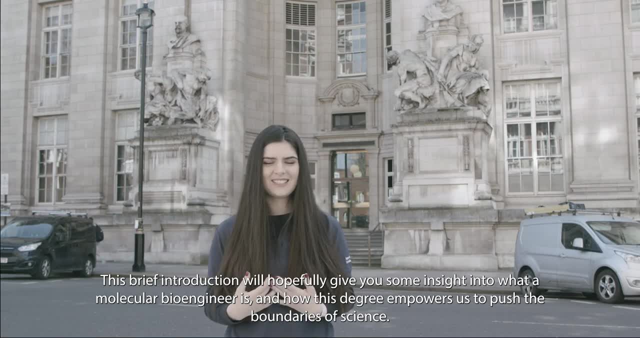 degree empowers us to push the boundaries of science. I'm now in front of the Royal School of Mines, which is where most of our lecture will take place. This is where most of our lecture will take place. This is where most of our 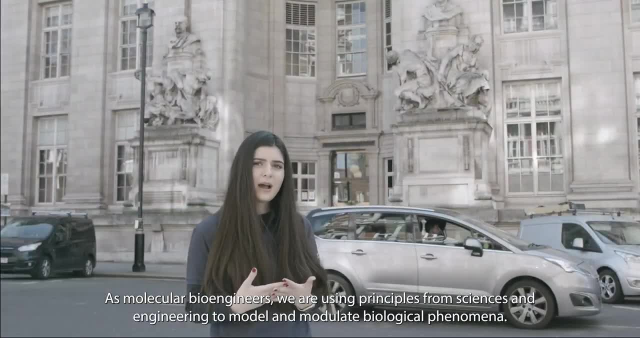 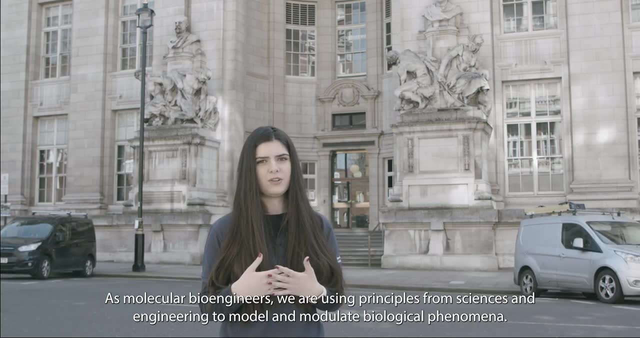 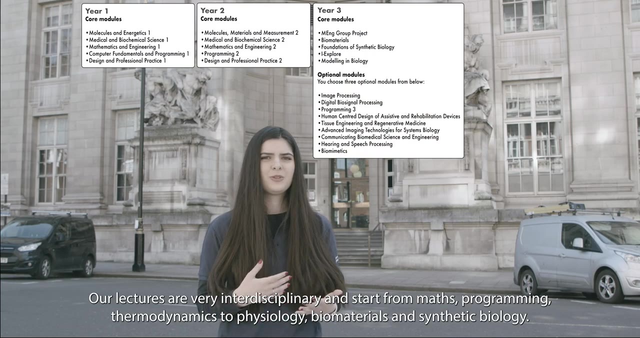 lectures will take place in normal times. As molecular bioengineers, we are using principles from sciences and engineering to module and modulate biological phenomena. Our lectures are very interdisciplinary and start from maths, programming, thermodynamics to physiology, biomaterials and synthetic biology. 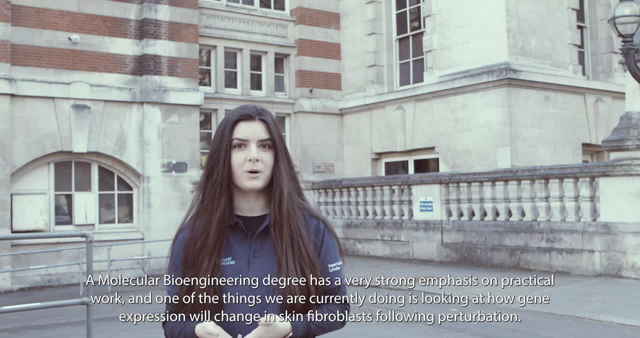 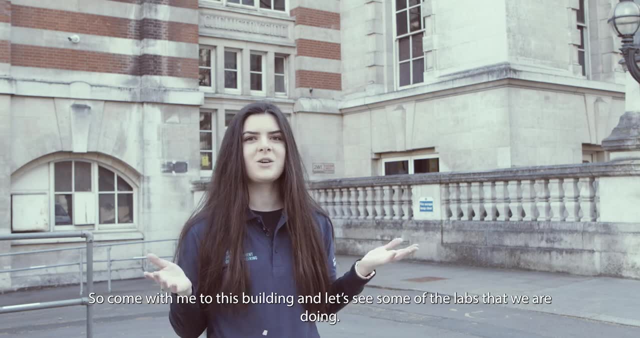 A molecular bioengineering degree has a very strong emphasis on practical work, and one of the things we are currently doing is looking at how gene expression will change in skin fibroblasts following perturbation. So come with me to this building and let's see some of the labs that we are doing. 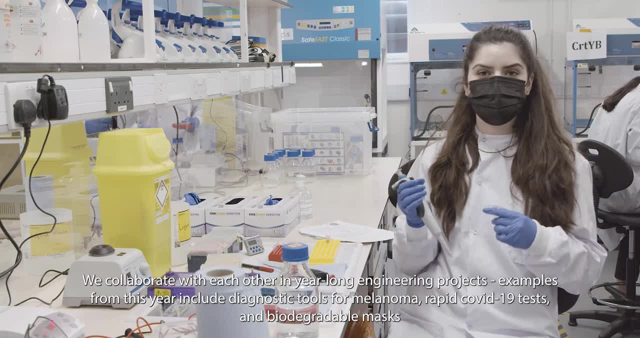 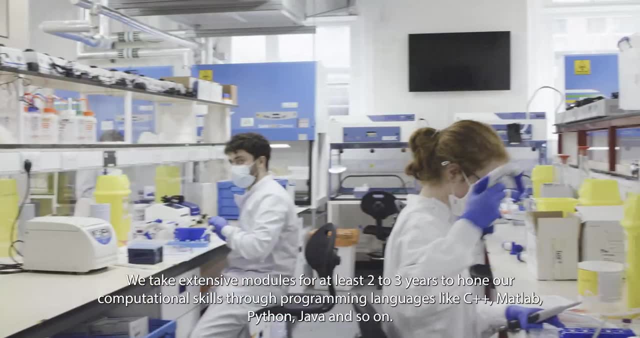 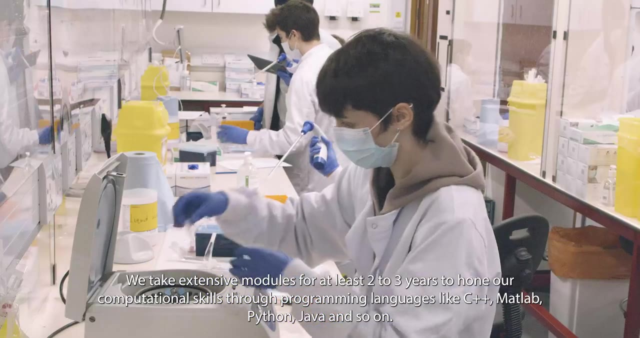 We collaborate with each other in year-long engineering projects, and examples from this year include diagnostic tools for melanoma, rapid COVID-19 tests and biodegradable masks. We take extensive modules for at least two to three years to hone our computational skills through programming languages like C++, MATLAB, Python, Java and so on. 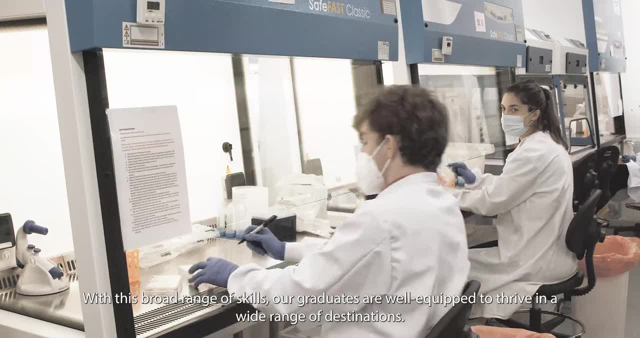 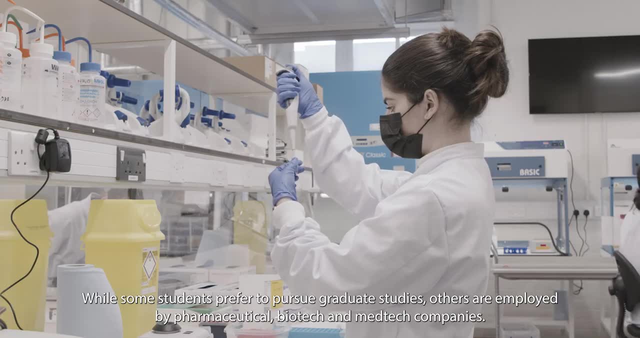 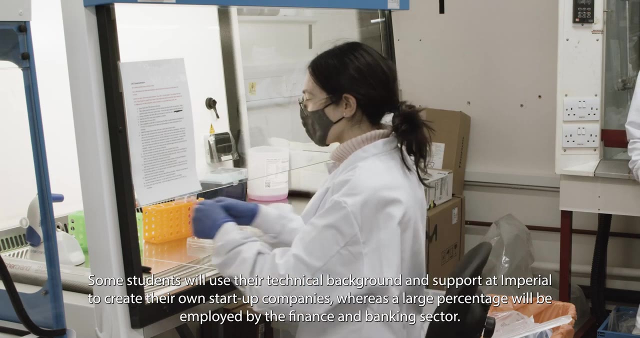 With this broad range of skills, our graduates are well equipped to thrive in a wide range of destinations. While some students prefer to pursue graduate studies, others are employed by pharmaceutical, biotech and medtech companies. Some students will use their technical background and support at Imperial to create their own startup companies, whereas a large percentage 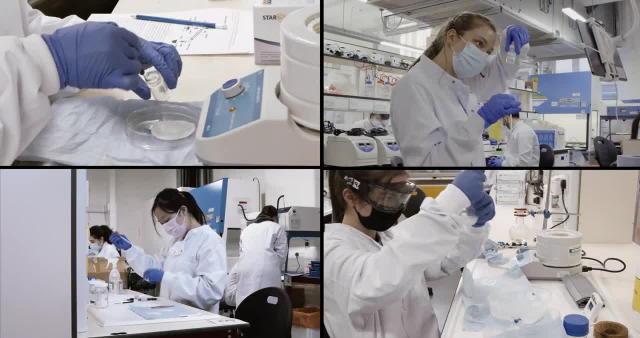 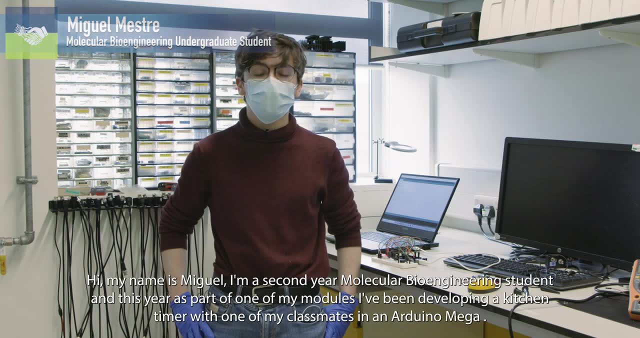 will be employed by the finance and banking sector. Hi, my name is Miguel. I'm a second year molecular bioengineering student at the University of Toronto. This year, as part of one of my modules, I've been developing a kitchen timer with 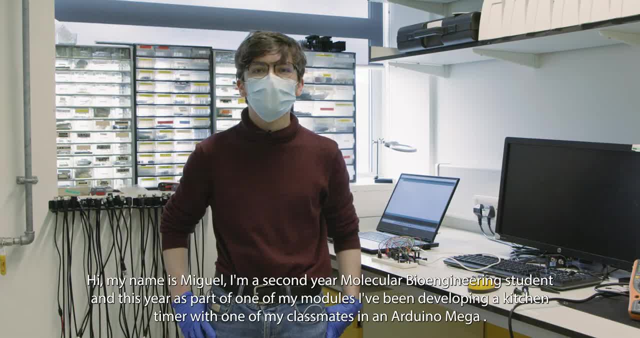 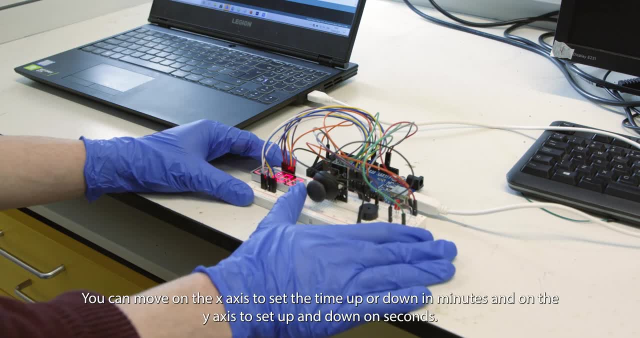 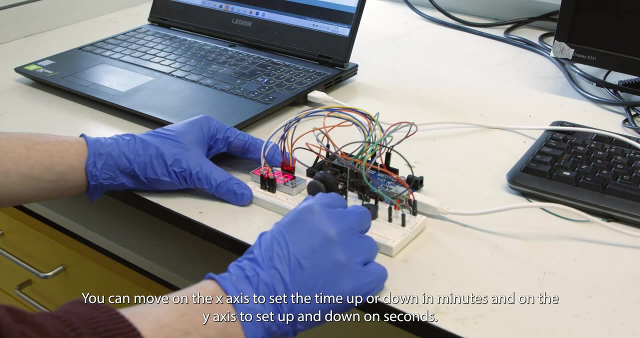 one of my classmates in an Arduino Mega. Our kitchen timer uses a 4x7 segment display and a joystick where you can set the time. You can move on the x-axis to set the time up or down in minutes and on the y-axis to 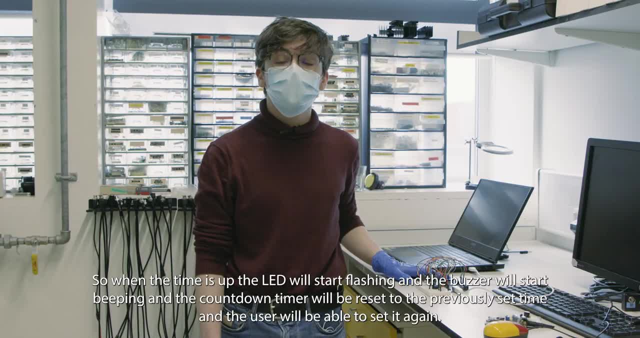 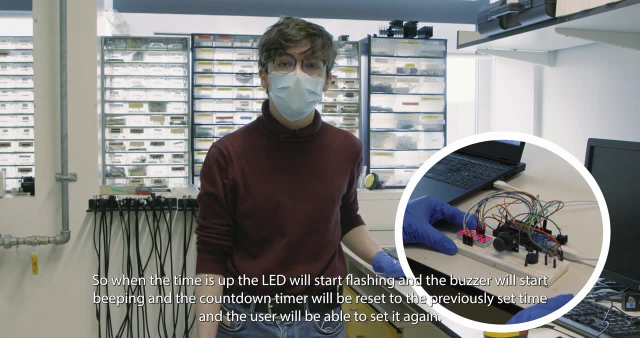 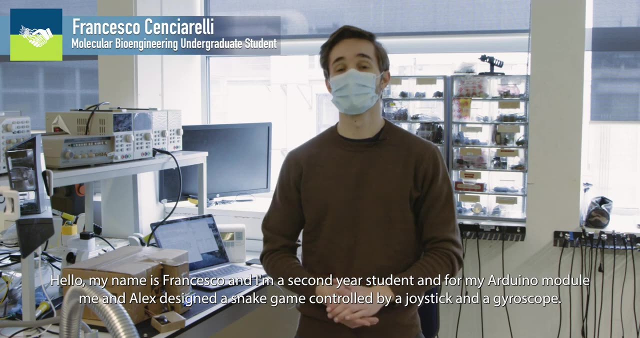 set up and down in seconds. When the time is up, the LED will start flashing, The buzzer will start beeping, The countdown time will be reset to the previously set time and the user will be able to set it again. Hello, my name is Francesco and I'm a second year student. For my Arduino module, me and. 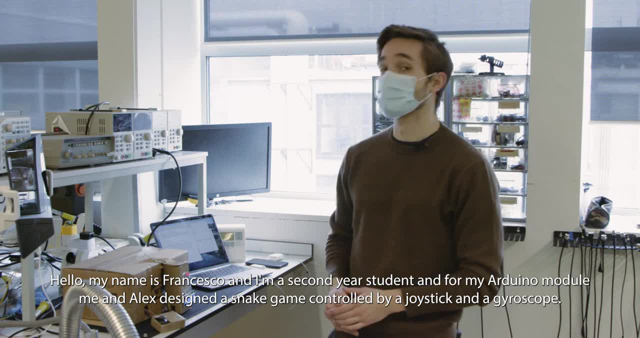 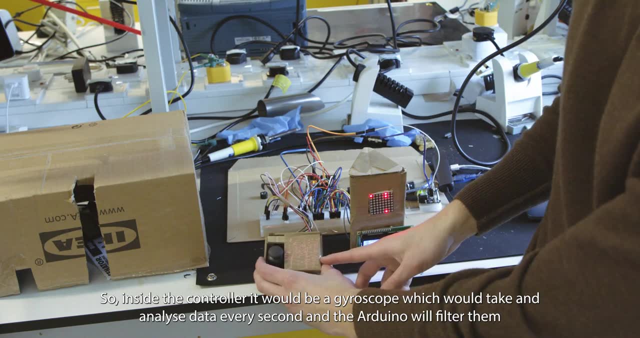 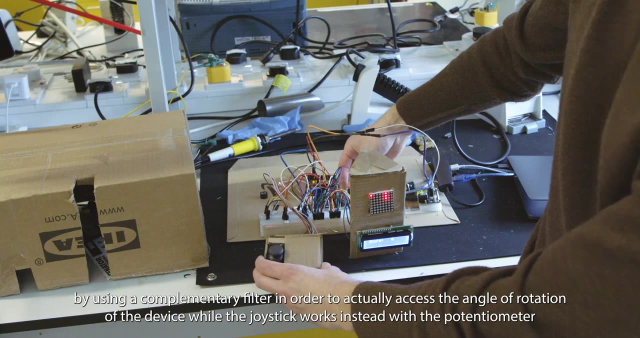 Alex designed a snake game controlled by a joystick and a gyroscope. Inside the controller there will be a gyroscope which will take and analyze data every second. Arduino will filter them by using a sensor. The gyroscope will use a complementary filter in order to actually access the angle of rotation. 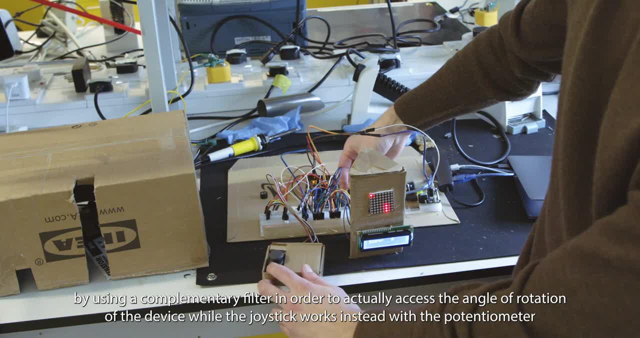 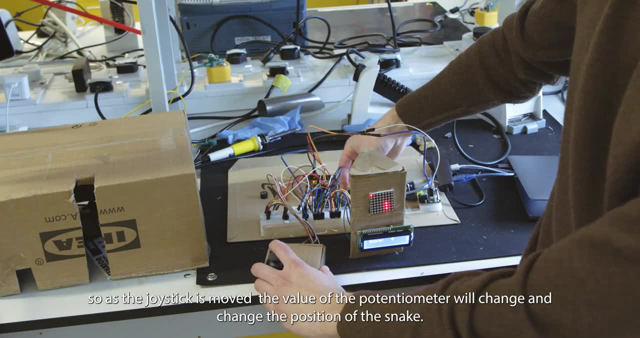 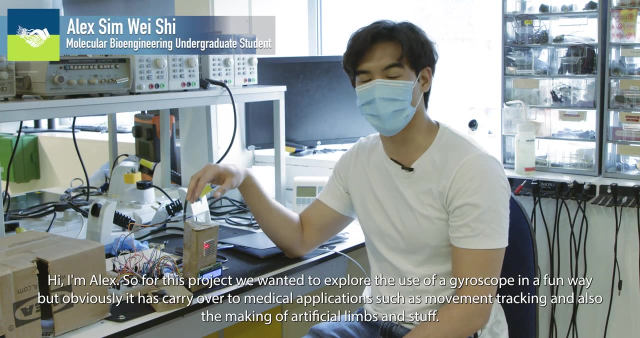 of the device, while the joystick works instead with potentiometers. As the joystick is moved, the value of the potentiometer will change and change the position of the snake. Hi, I'm Alex For this project. we wanted to explore the use of a gyroscope in a fun 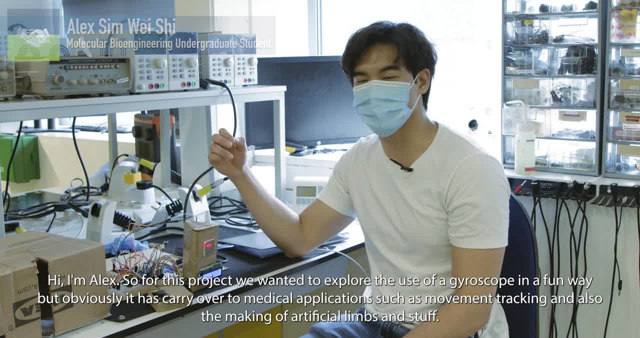 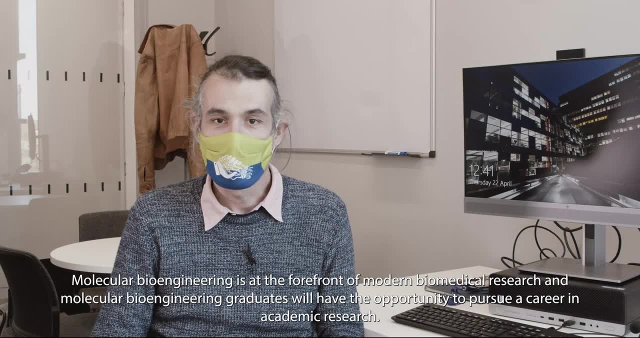 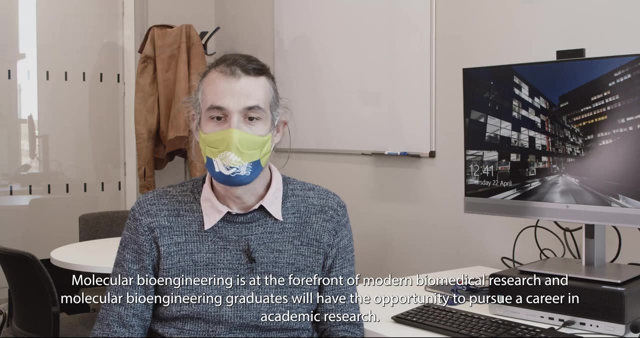 way, but obviously it has carryover to medical applications such as movement tracking and the making of artificial limbs itself. Molecular bioengineering is at the forefront of modern biomedical research, and molecular bioengineering graduates will have the opportunity to pursue a career in academic research In 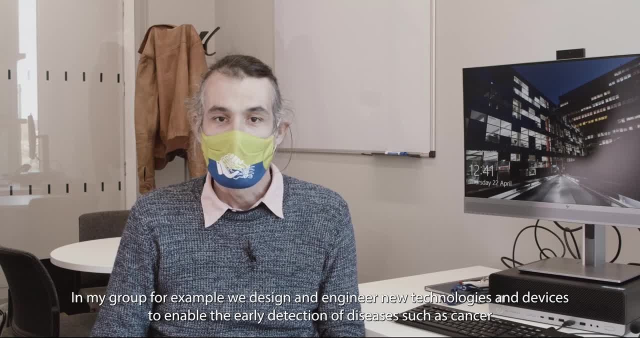 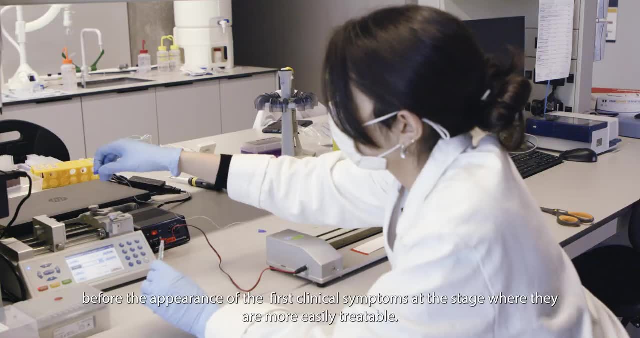 my group, for example. we design and engineer new technologies and devices to enable the early detection of diseases such as cancer before the appearance of the first clinical symptoms, at a stage where they are more easily treatable. This is mostly done via the detection of biomarkers or indicators. 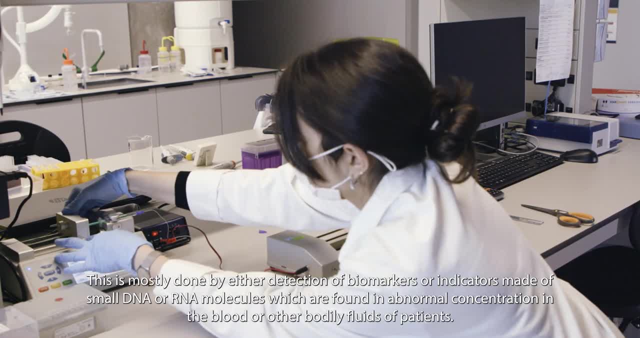 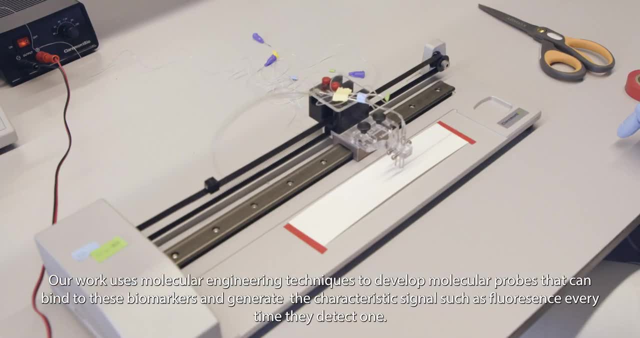 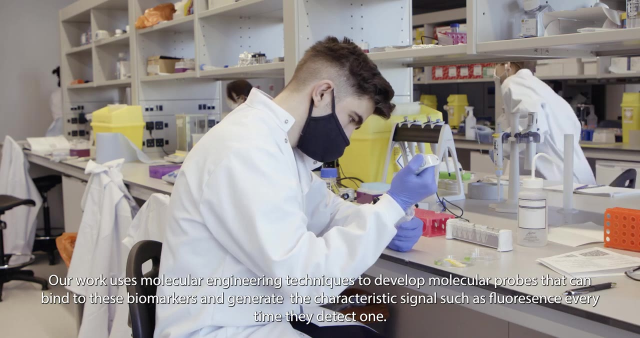 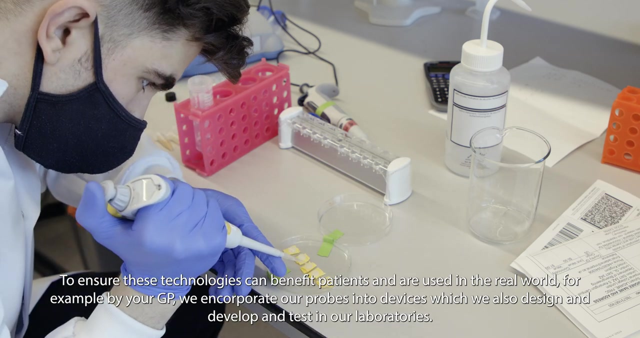 Our work uses molecular engineering techniques to develop molecular probes that can bind to these biomarkers and generate a characteristic signal, such as fluorescence, every time they detect one. To ensure these technologies can benefit patients and are used in the real world, for example by your GP, we incorporate our probes into devices, which we also design, develop and.